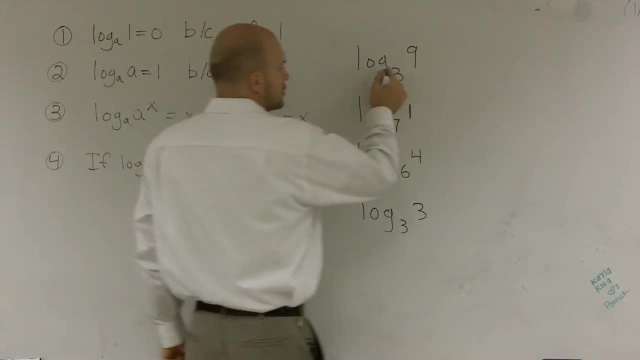 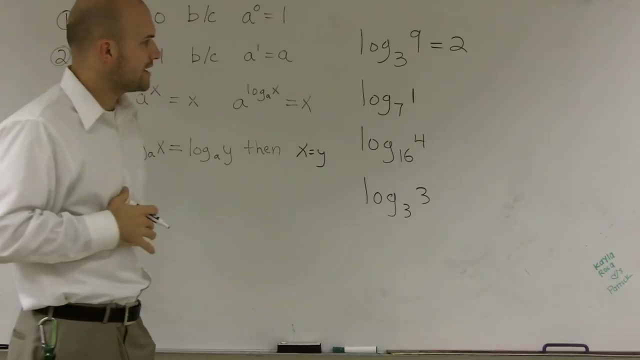 basic one You could say. well, the answer to that is: obviously we know it's going to be 2.. Log base 3 of 9 is 2. Because I can multiply 3 by itself twice to get me 9.. Now here I have log base 7 of. 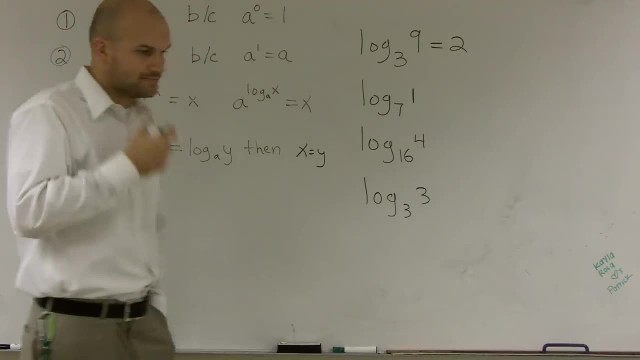 1.. So 7 raised to what number gives me 1?? Now, if you're very familiar with your exponents, you could say: oh well, that's going to be 0, because 0 raised or 7 raised to the 0. 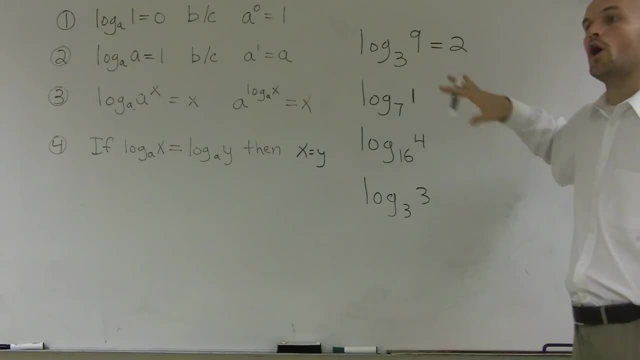 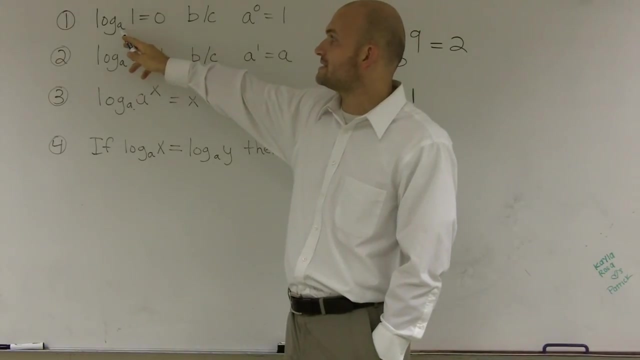 power gives me 1.. And what you'll find out is- that's actually true for all logarithms and all numbers- that any time it doesn't matter what our base is, any time we raise it, or whenever we have our base and we're you know we're going to have a logarithm. 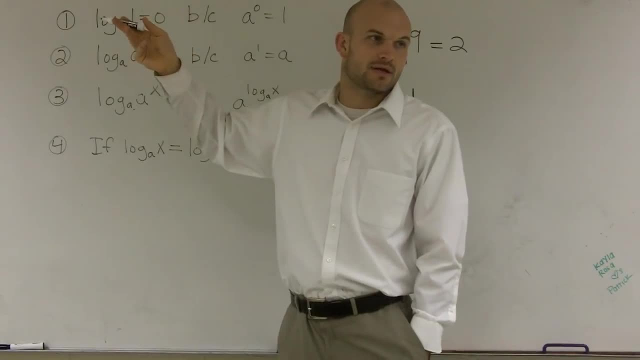 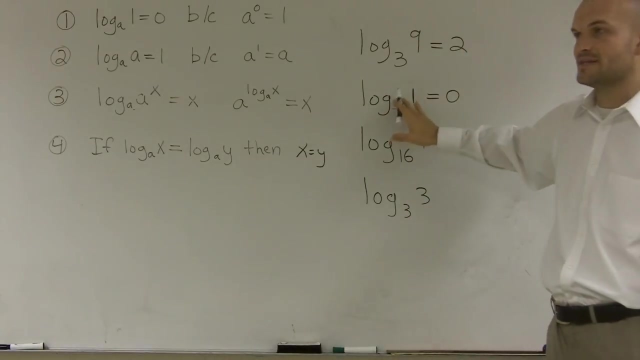 and we evaluate it for the logarithm of 1, it's always going to equal 0, right, So this answer is going to equal 0. Whenever you're taking the log, it doesn't matter what the base is of 1, it's going to equal 0.. Here we have a base that's larger than what we're. 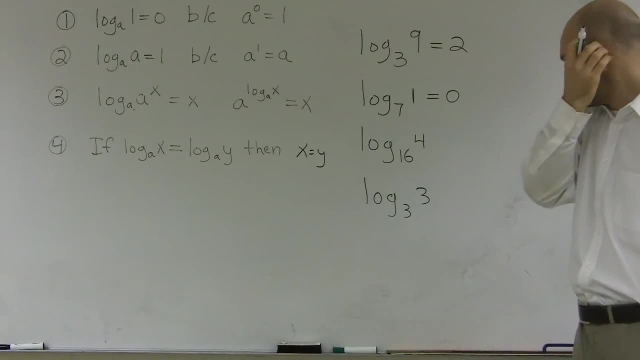 evaluating for. So we need to start thinking about this and say: well, if 16 was raised to the first power, it'd be 16.. If 16 were raised to the second power, it'd be 16 times 16, which is greater than, which is going to be greater than 16 times 16.. So we're going. 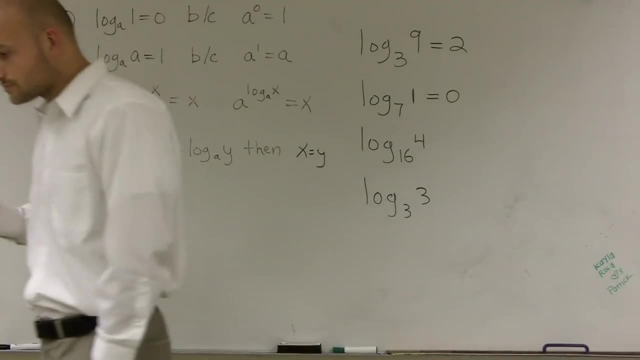 to need to think of a number that is going to be greater than, you know, 16.. I'm sorry, that needs to be less than 16. And so that, therefore, my exponent has to be smaller than 1. So I'm going to have to be dealing with a fraction And a couple ways to kind of think. 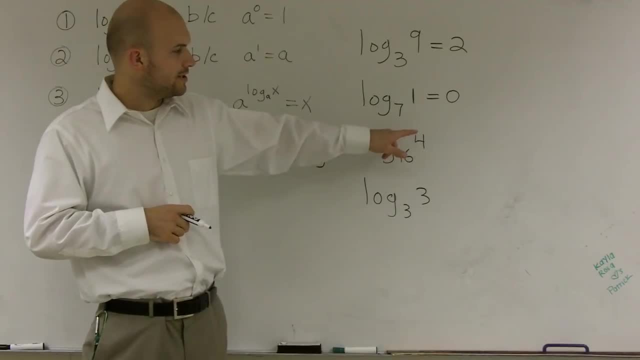 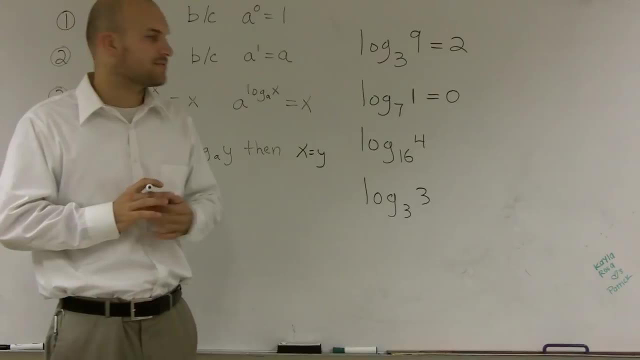 about this is well. one thing I notice is: you know 4 and 16, how are those related? Well, you know, 16 is the square root of 4.. How else can I write the square root? I'm sorry, 4 is the square root of 16.. How else? 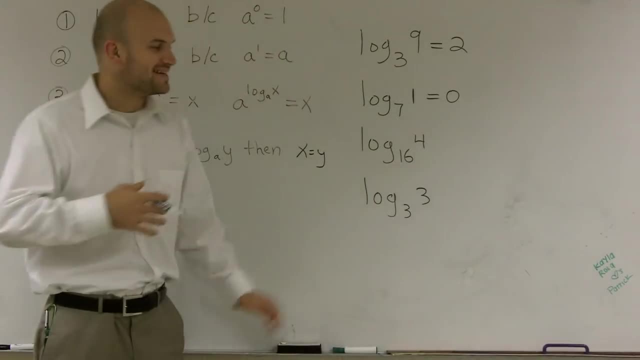 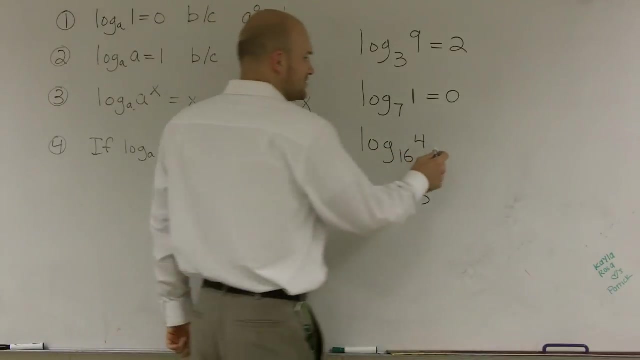 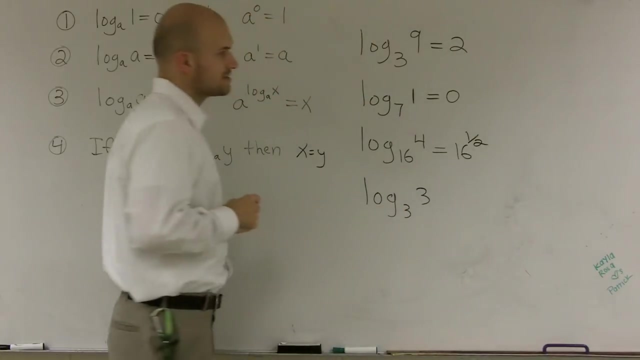 can I write 16?? Or 16 is the square root of 4.. How else can I write the square root of 16?? Well, you could also write it as 16 to the 1 half power, 16 to the 1 half power. 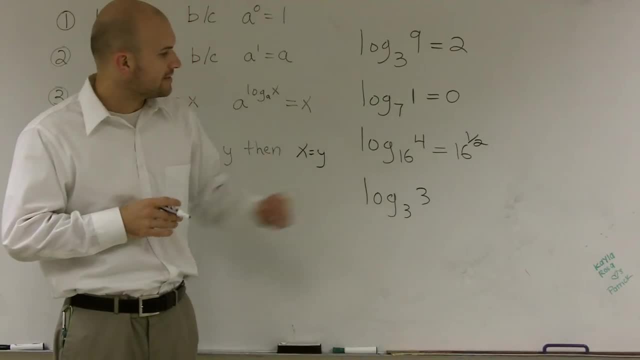 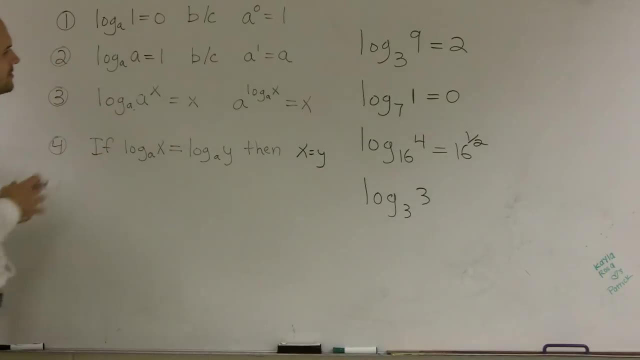 is going to be the square root of 16,. OK, Then last problem I'm going to do is do log base 3 of 3.. So, to do log base 3 of 3, what you need to look at again, I'm going to look.